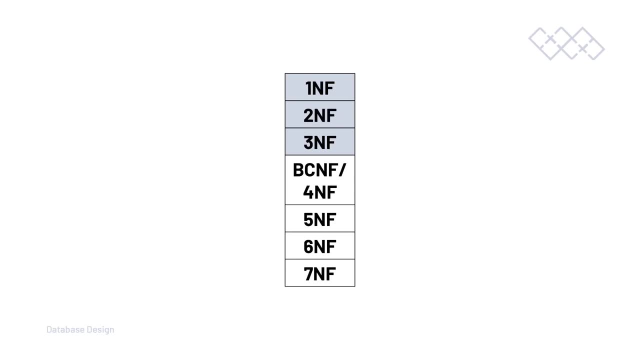 sometimes very quickly arrange our fields and tables into third normal form. now your table and fields can only be in third normal form or second normal form, etc. if they meet the standards of that particular normal form and all the other standards and rules below that. so if i want to, 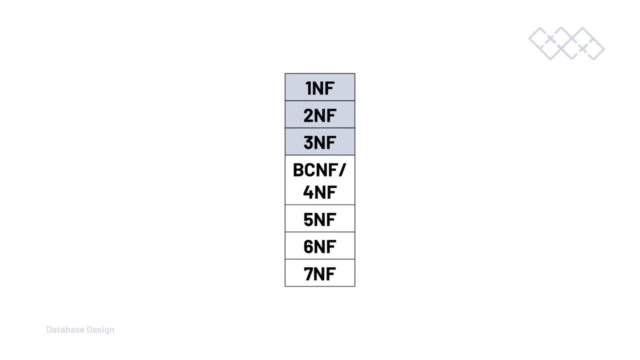 get my tables into third normal form, i need to make sure that they are meeting the standards and rules of the third normal form, second and first normal form. so typically we aim to develop our database design into at least the third normal form. we might refer to this as the operational. 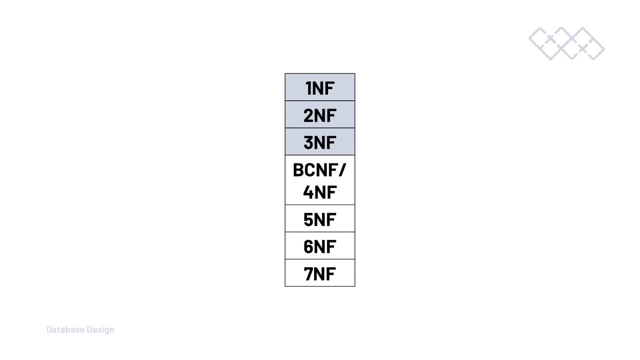 level. now, for various reasons related to performance trade-offs, it is not always considered beneficial to normalize further. in this course we aim to get our database design into third normal form, so we work through the normalizer process in order to reduce redundant data, repeating data that might be within our database. 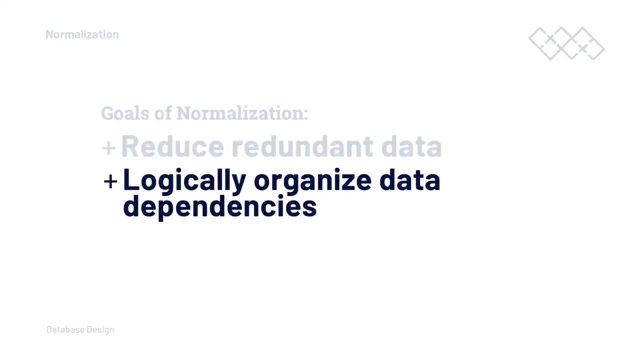 tables. the normalization process also encourages us to think about how our attributes and fields relate to each other- so dependencies- and steers us towards having only related data in a table. ultimately, this all leads to helping to protect the integrity of the data that we store in our 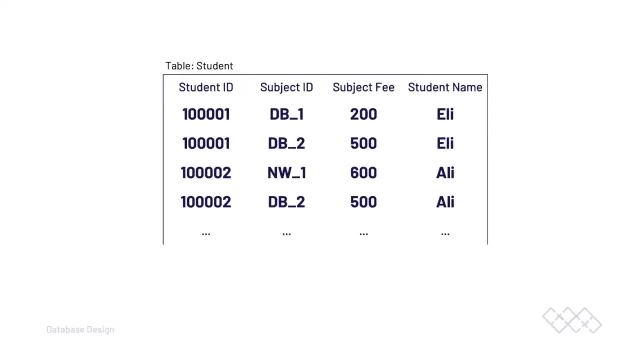 table. once you understand the normalization process, you will quickly spot potential redundancy and dependency issues within the table. one of the recommendations i make is that, when you're trying to find redundancy and dependency issues, that you try and model your data in a table and that will give you a better view of your data and identifying these potential issues. 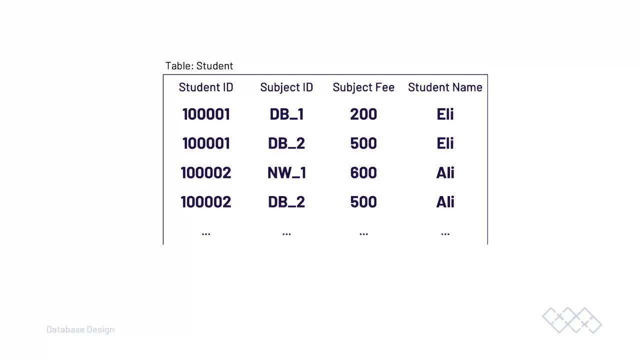 taking a look at this table here. there are a few different occurrences here and i'm going to go back into the live slides segment and see how you can figure out which questions we shouldn't go into option one. نجمعی's first factor is number of questions. 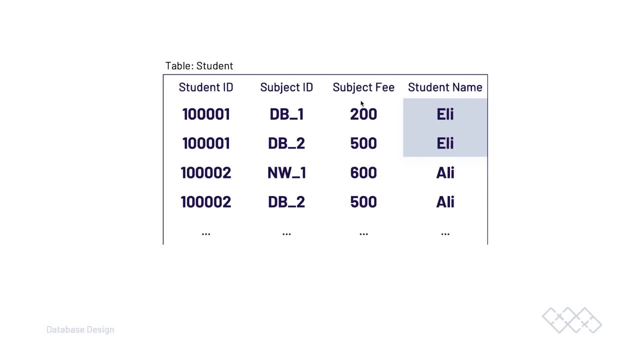 that are being asked and it's the المست principe that serves the purpose of conducting the heading grouplaud. chromed ID analysis and accuracy analysis of relevant data is being copied twice, so we have some more redundant data. so ideally we're trying to remove that and only specify the subject fee once for, in this case, a particular subject. 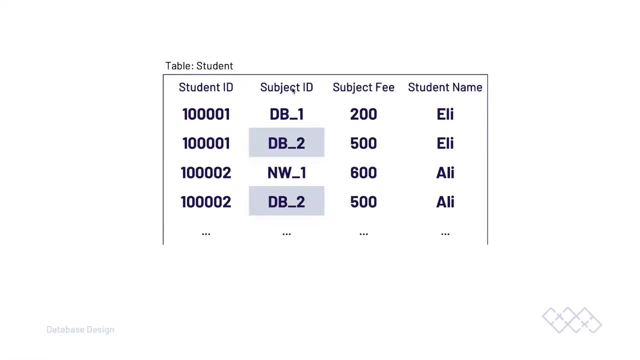 of course we're repeating the subject fee, so potentially we are repeating information about the actual subject. now let's imagine we wanted to, for example, update this subject database to the amount it costs. in our database we might have multiple occurrences of this. so if we were to update this subject fee to maybe 600, we would have to do that for. 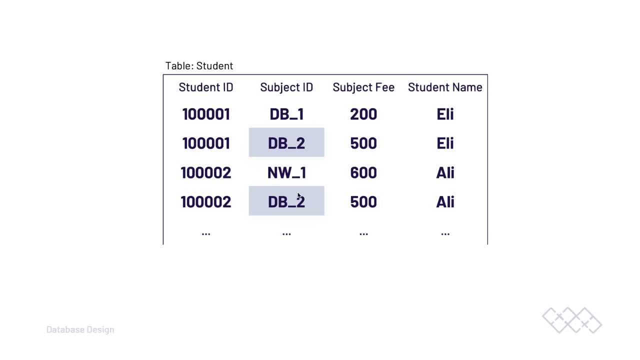 every single field of that instance and that's where potential errors errors, that's where potential errors occur. and then, last of all, you can see there are some redundancy issues here that looks like we're repeating information about the student, as we previously saw. so the normalization process is going to allow us to remove some of those or at least reduce. 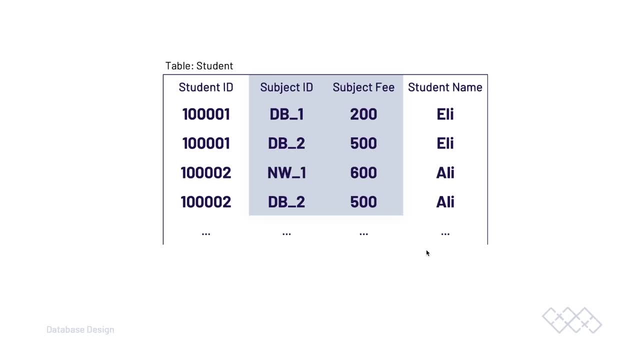 the number of errors that we have in our database, so we're going to remove some of the amount of redundant data. now, dependency is a little bit harder to explain and we will move through this in this course and i will give you a better understanding of dependency. 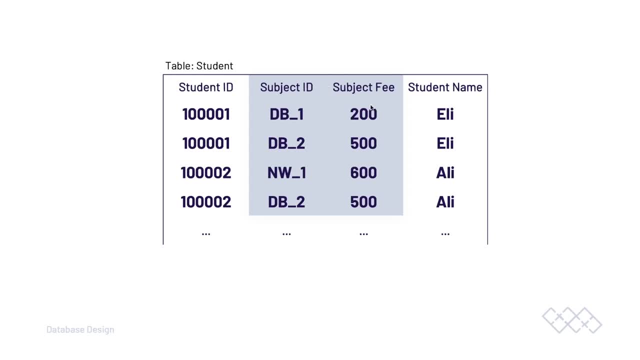 but here what we have is the subject fee. how can we determine how much the subject costs? but we do that by i first of identifying, for example, the subject id. so if i would, if i were to know the subject id, then i can then determine from this table, from this row, the subject fee. 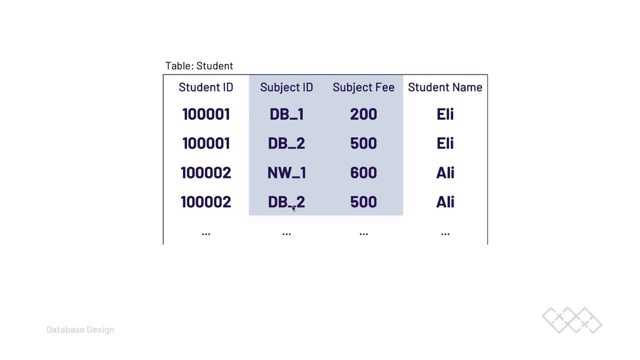 so we can see that database two. anytime there's database two you can see that the numbers are the same. so we can say that the subject fee is dependent upon the subject id. now one of our goals to move into the third normal form is to make sure that all the attributes here will be: 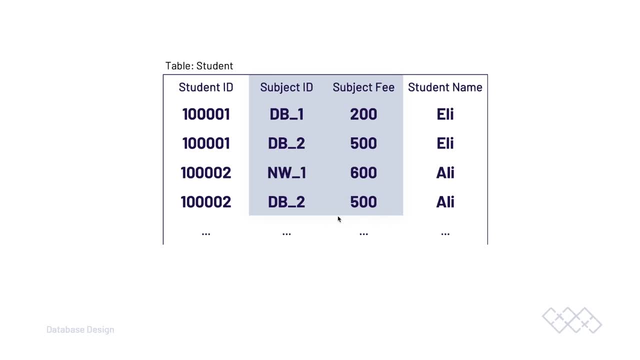 associated or dependent upon what will be known as the primary key, and in this instance, that's not going to be true, potentially so. there's something that we need to do to remove this from this table, and by doing that, not only are we going to remove and resolve the dependency issue, but we will also.